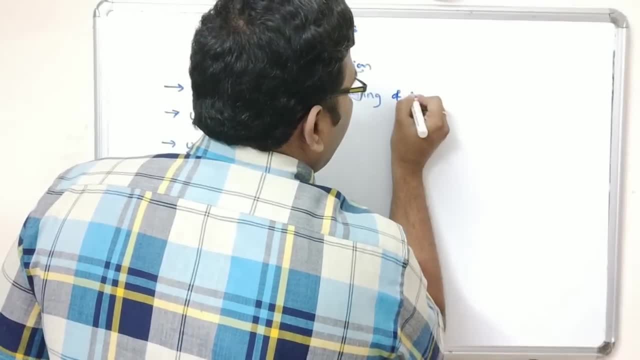 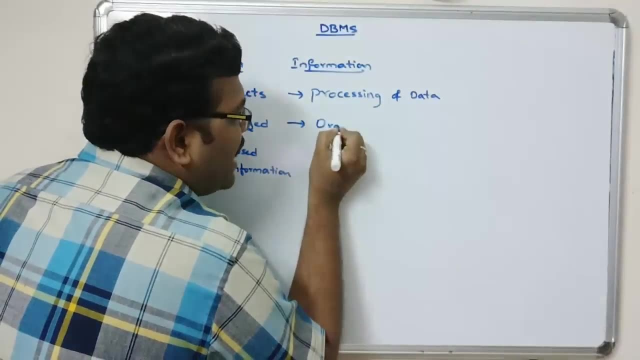 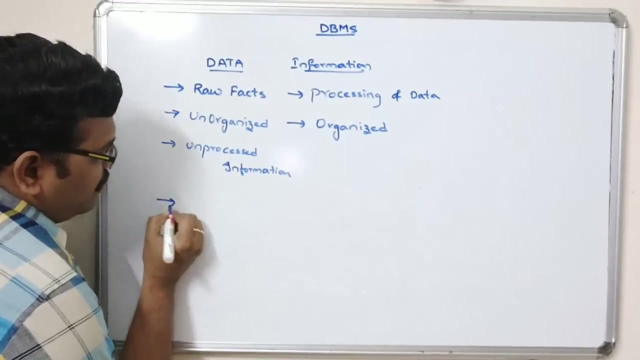 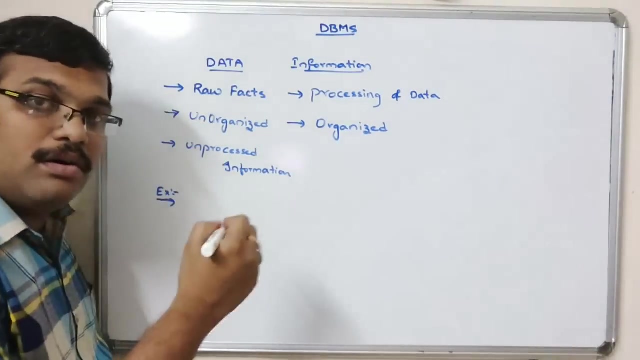 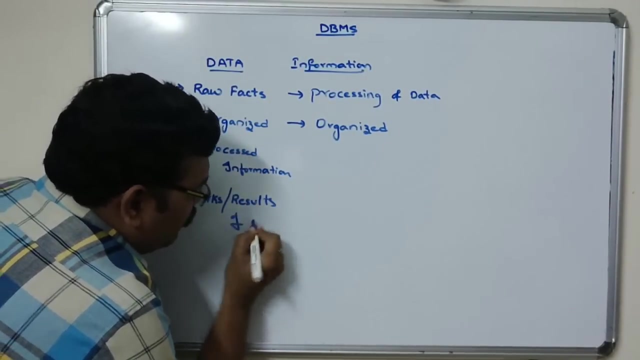 is a processing of data, So after processing the data will get the information right. So this will be important information. Beta and alpha have different methods of 발생: organized fashion, organized for example. for example, so if a class consists of a 60 students, the information or the marks or the results, so complete class or 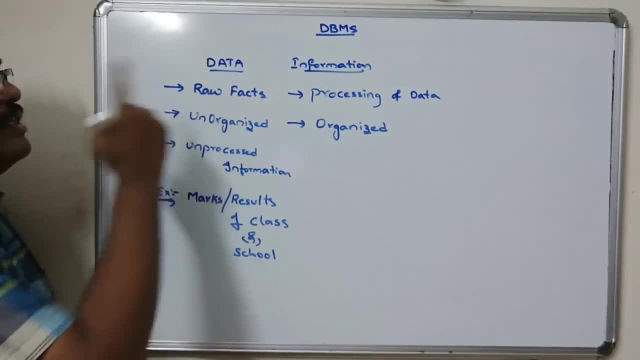 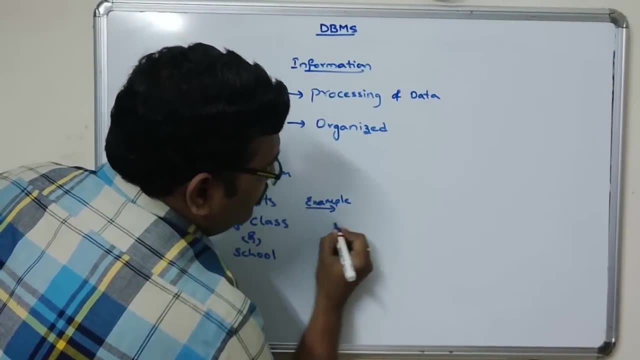 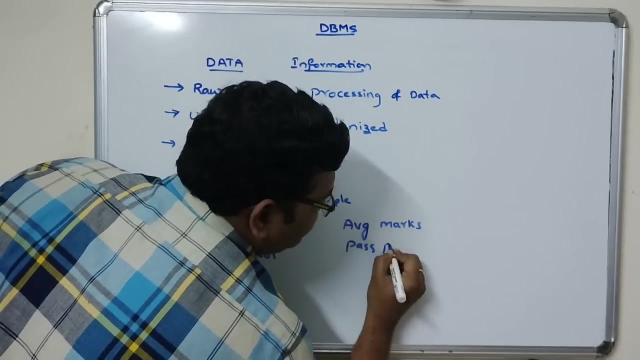 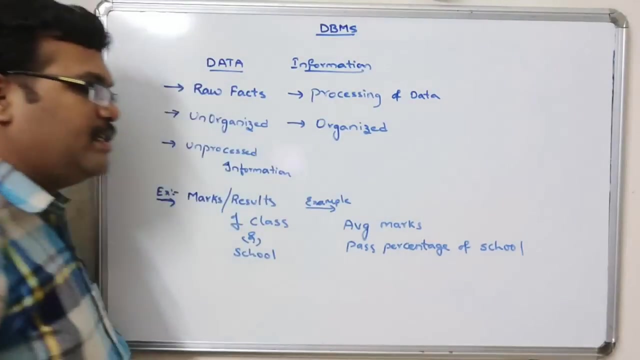 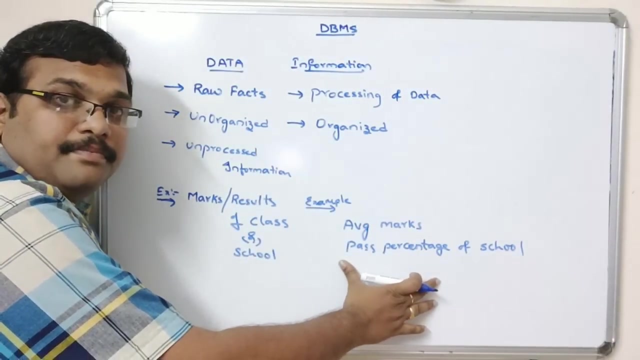 school or college will comes under this data and here example we can say the average marks or the five percentage. the past percentage of school or college is called information. that means the complete data and the information right. so after processing the data will get the information right now. 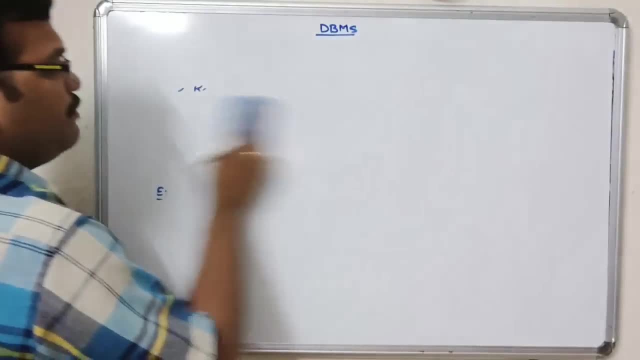 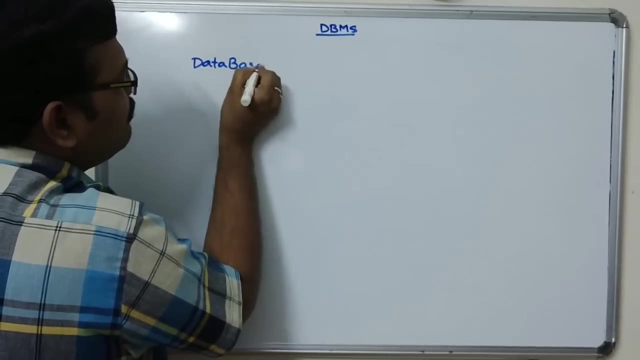 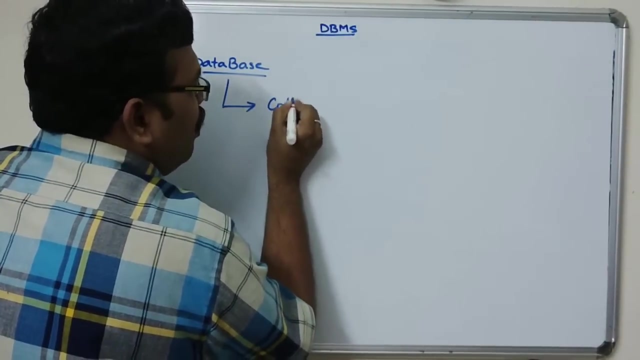 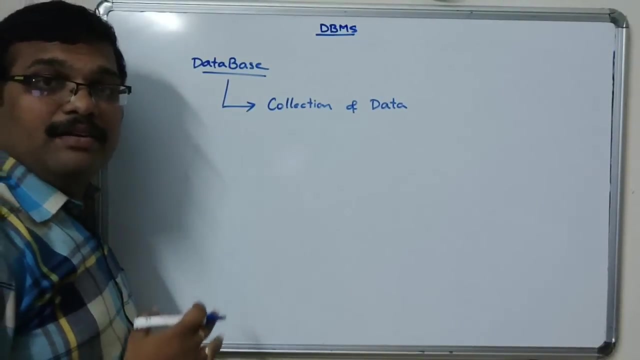 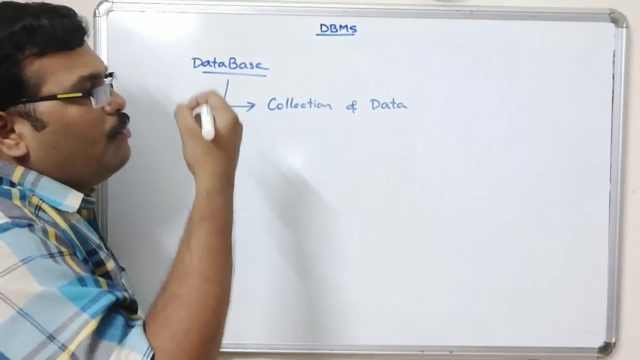 here our subject is: what is our subject? that is dbms. dbms means database. so first, database. so what is meant by this database? so database means the collection of data, collection of data. so the database will be very large or very high right. so from that database we have to retrieve the data. that means this database will be having a large. 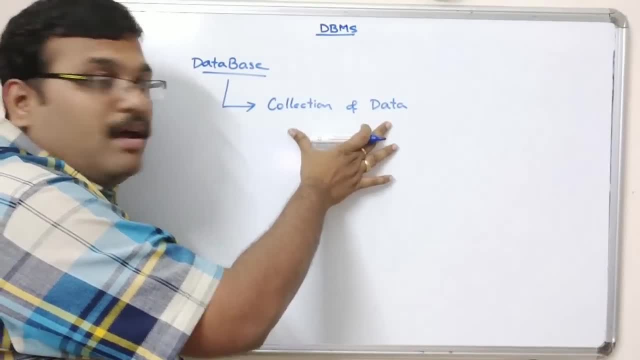 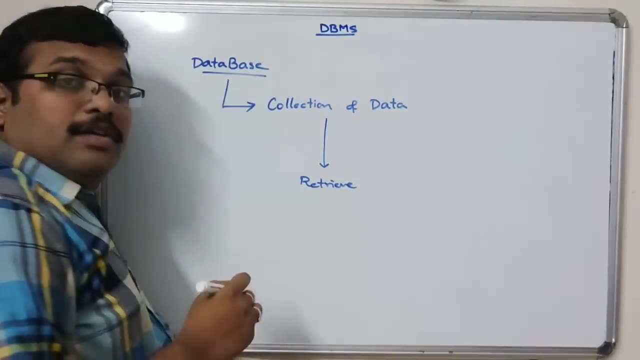 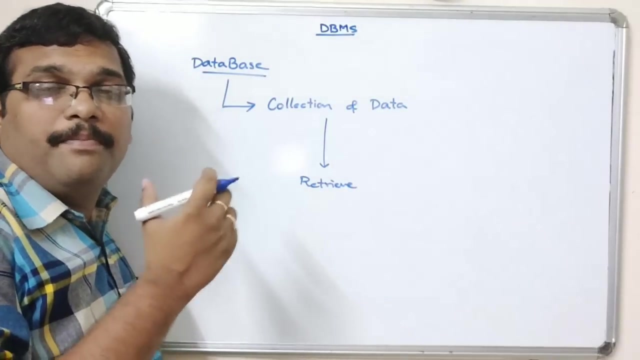 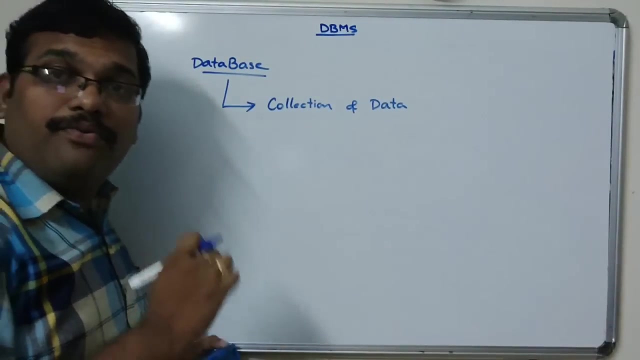 amount of data and from this data we have to retrieve right. so we'll create the data and we'll retrieve the data based upon some of the data that we have collected, some information, or based upon some processing right. so this is called a database collection of data. so the objectives: 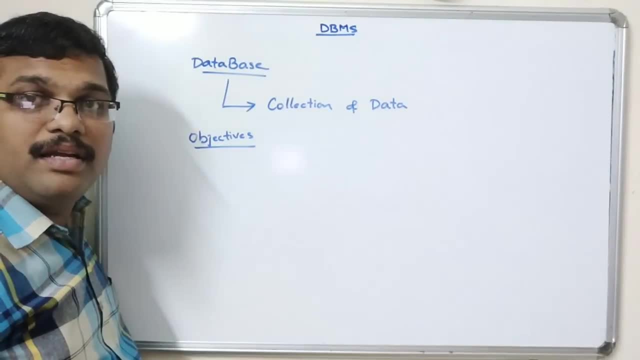 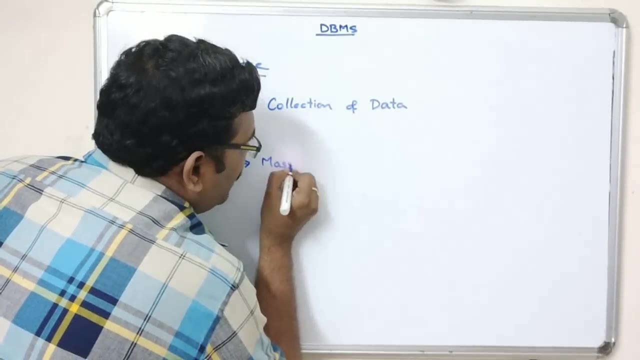 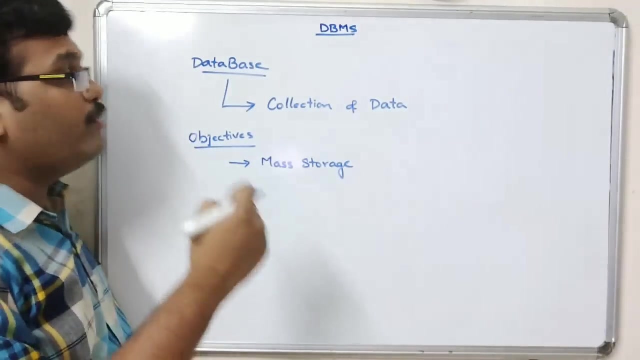 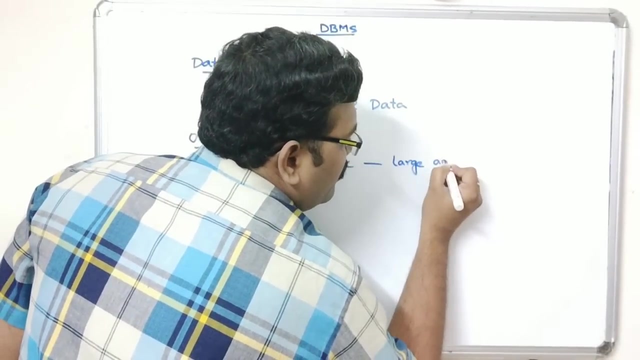 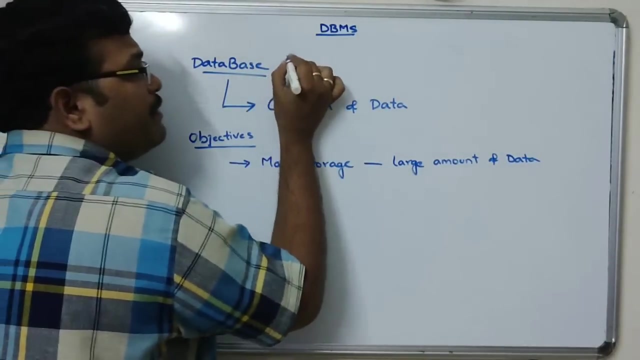 the main objectives of this dbms is the first one, the mass storage. so large amount of data can be stored at a single place. that we call it as database. so it can accept large amount of data. right, so this database can also be represented as db, db. wherever you see this db that we call it as. 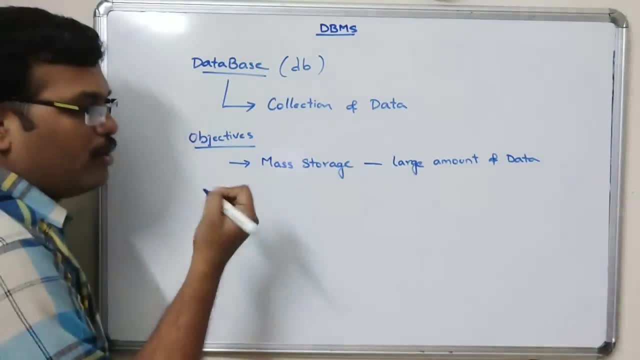 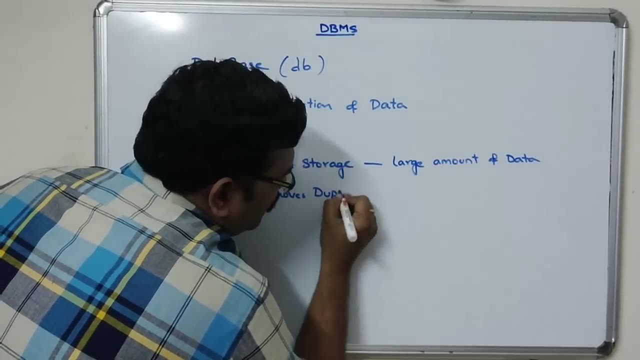 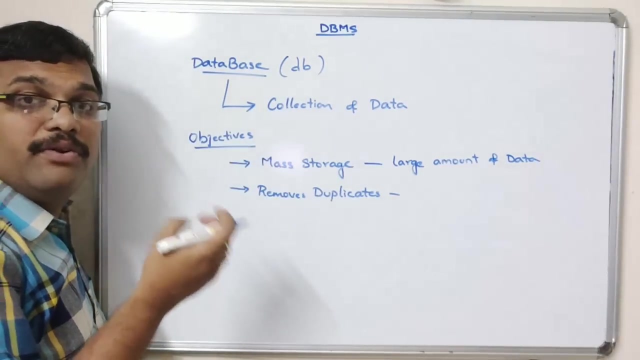 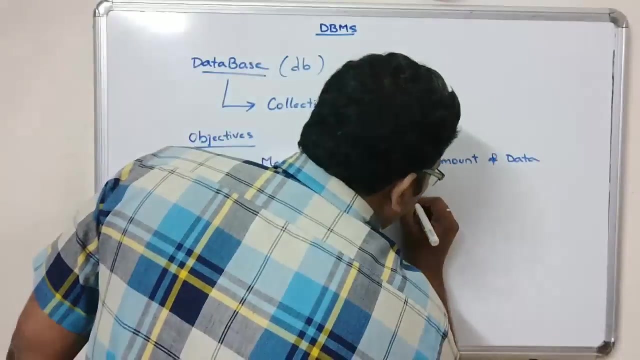 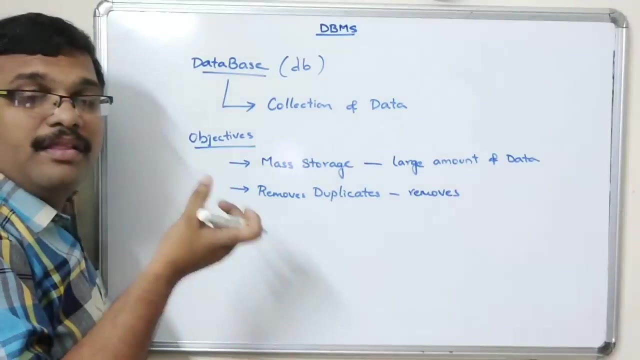 a database. okay, then there's a first objective. the next one removes duplicates. so this database is having an objective: that it can remove the duplicates if they occur right, it will remove all the duplicates. it removes all the duplicates so unique data can be maintained. the unique data that means without any. 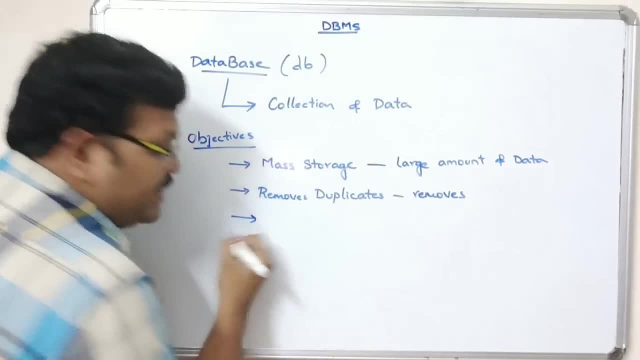 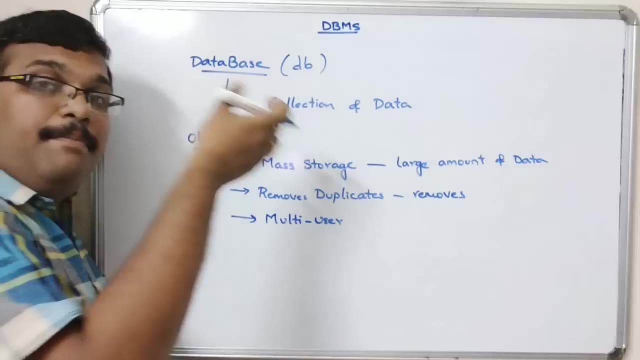 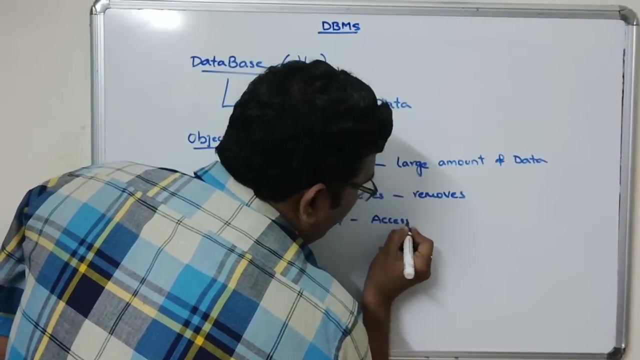 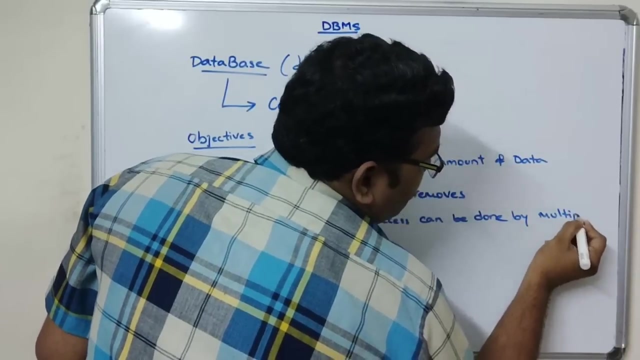 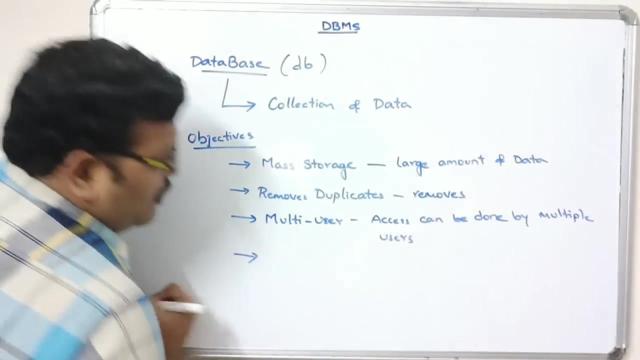 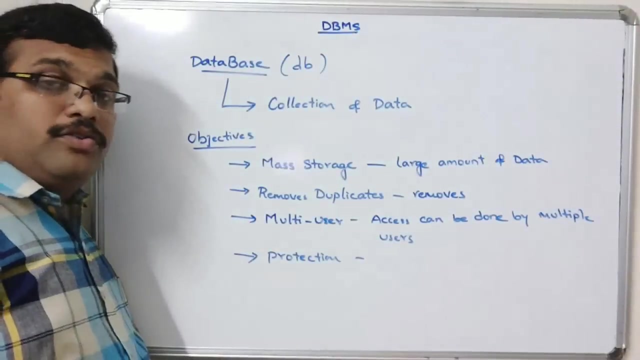 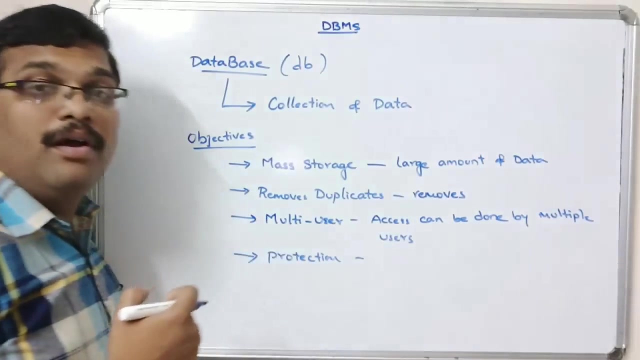 the data can be maintained. so the next one is multi user. so this database can be accessed by multiple users at a time right. so access can be done by multiple users. I will tell you an example for this. so and then protection. so in this database we can also secure the data. that means, the data can be secured with. 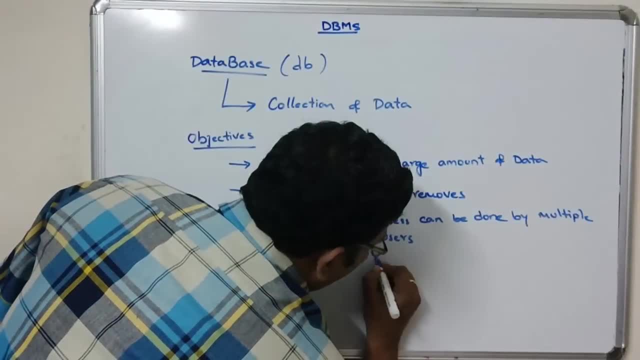 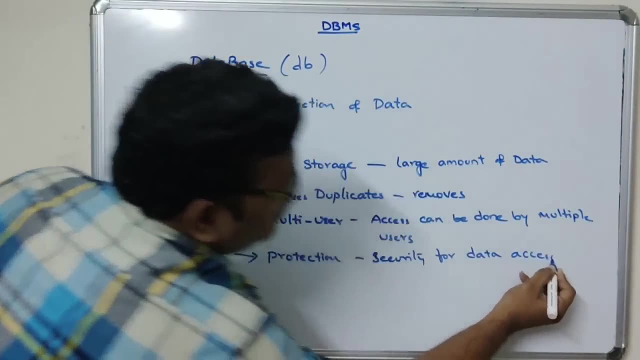 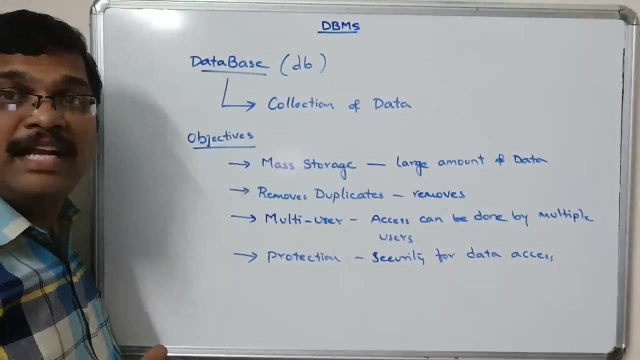 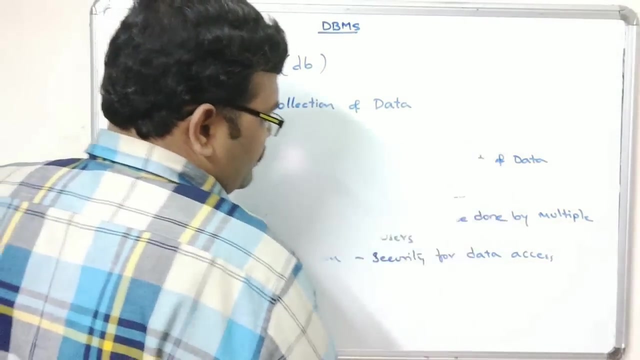 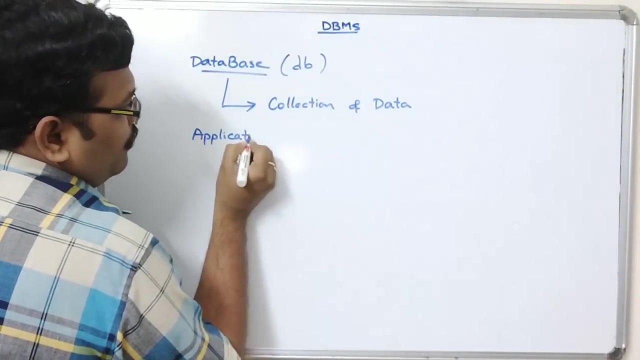 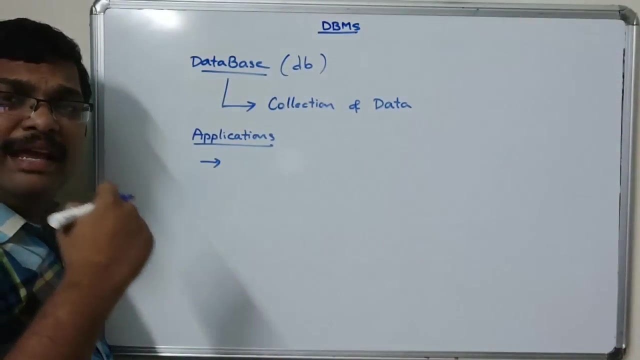 some restrictions, so providing the security for data access right. this can also be done in database. so these are some objectives of database management system. now where we have to use this database, so applications, the applications of DBMS, so we can use this DBMS in any application. 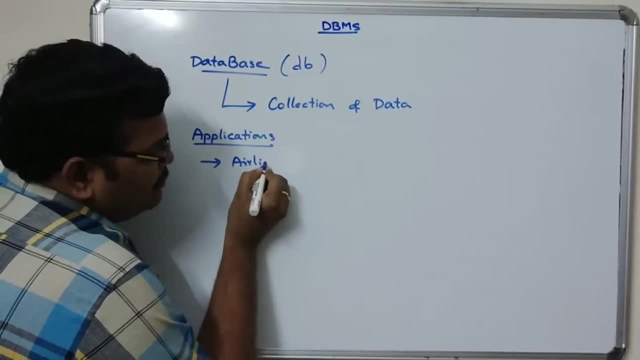 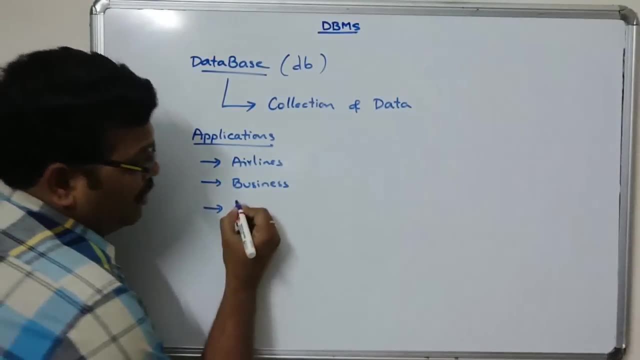 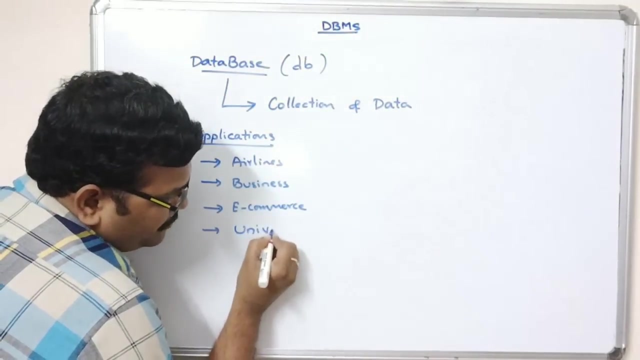 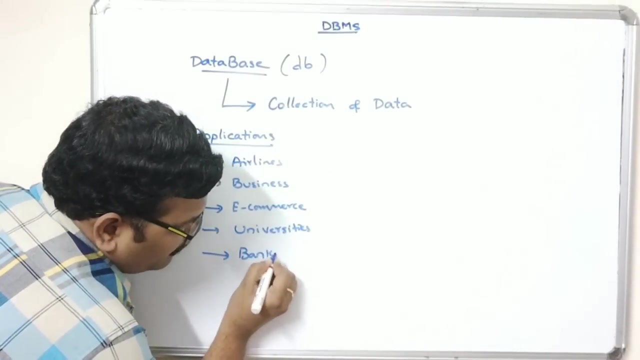 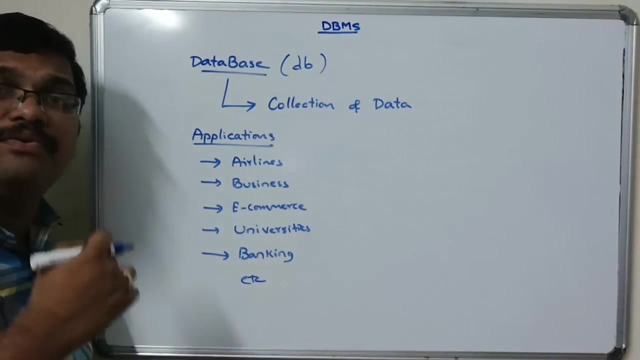 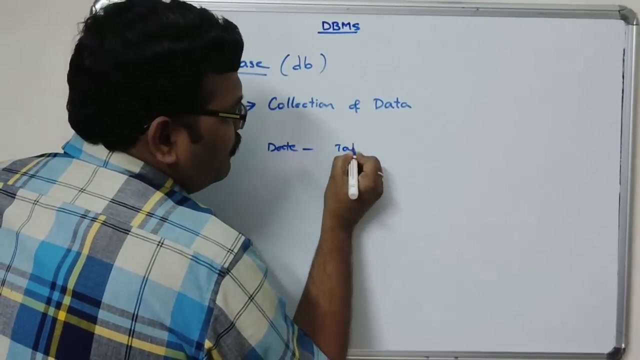 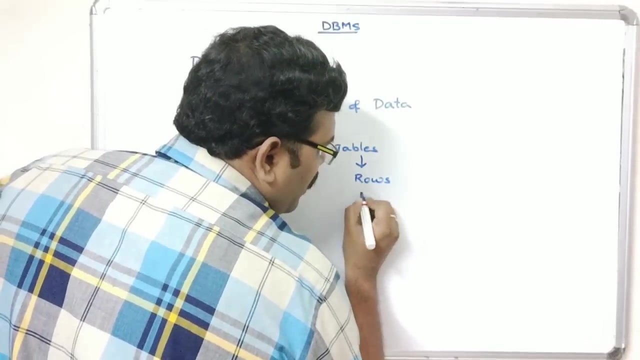 Like some: airlines, business, e-commerce, e-commerce sites, universities, banking- it's very important banking, so number of, etc. There are number of applications where we can use the database. Actually, here the complete data will be stored in the form of tables. In the tables there will be rows and columns. 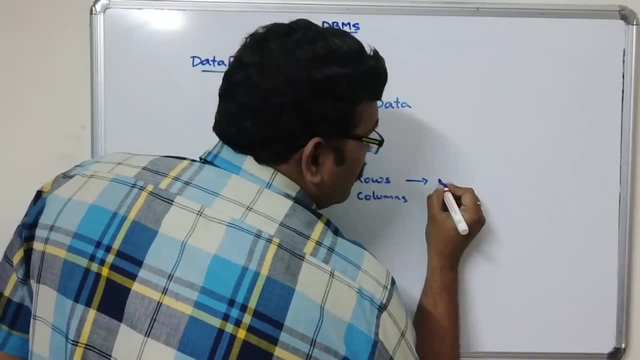 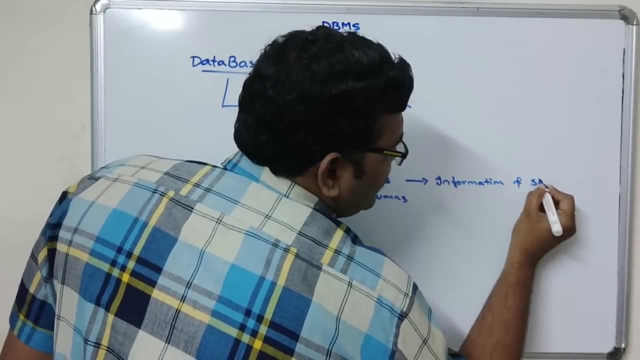 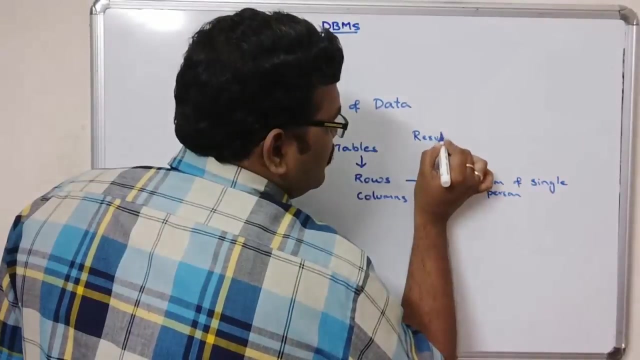 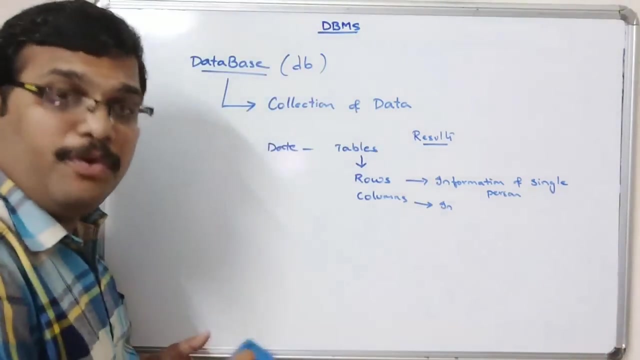 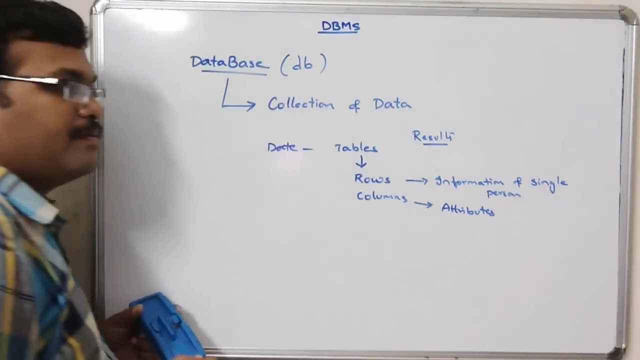 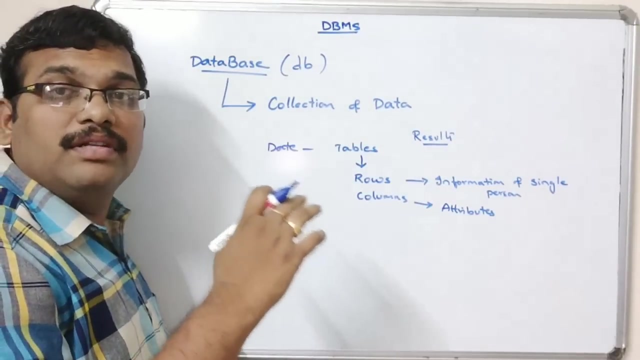 And rows are the information of a single database. Let us take an example for results. And columns are the information, or simply we can say attributes. Columns are attributes. So from this table the data will be retrieved and it will be displayed on the screen. 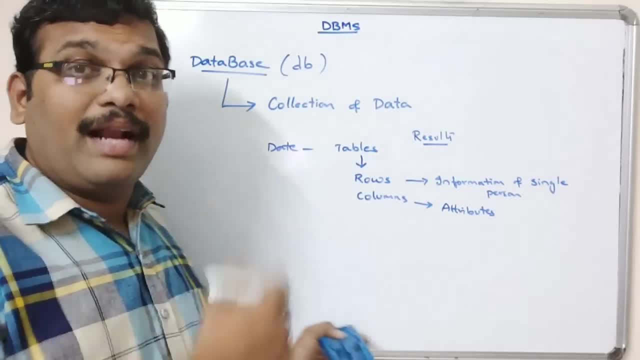 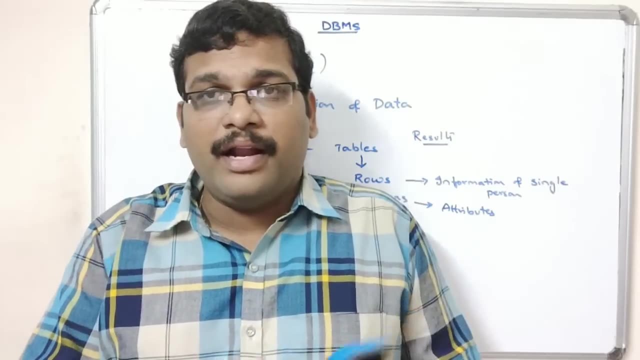 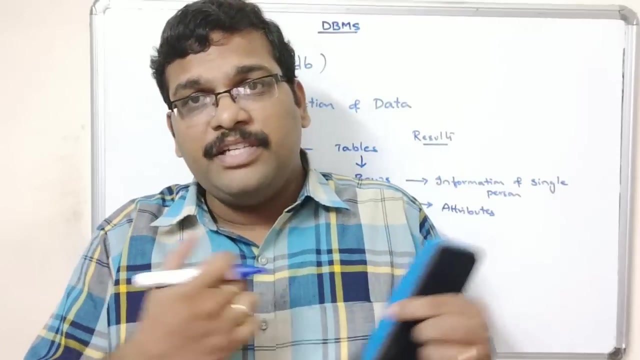 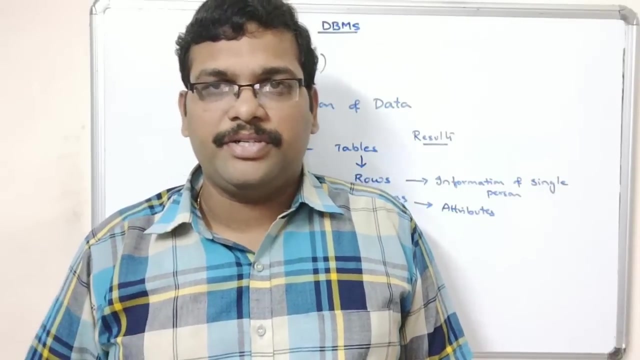 So this is called DBMS. That means organizing the data, the processing the data- So that's why I call it as a data is a unorganized or unorganized information and the information is an organized manner. That means we have to retrieve the data based upon some information. 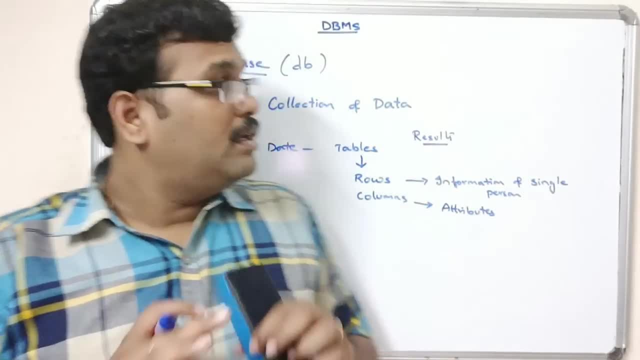 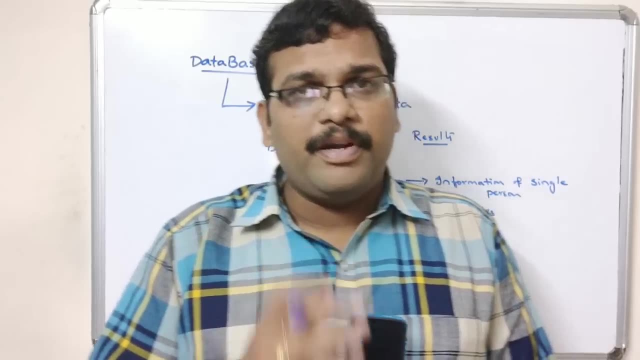 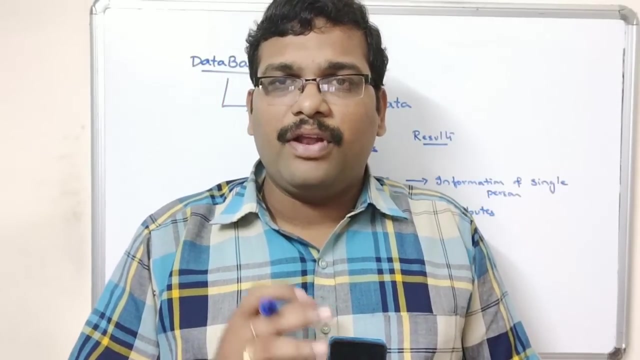 I mean some processing. So this is all about the introduction about the DBMS. So let's stop here, And In the next session we will go with the properties and the architecture of DBMS, Right? So thanks for listening And if you are having any doubts, you can feel free to post your doubts in the comment section. 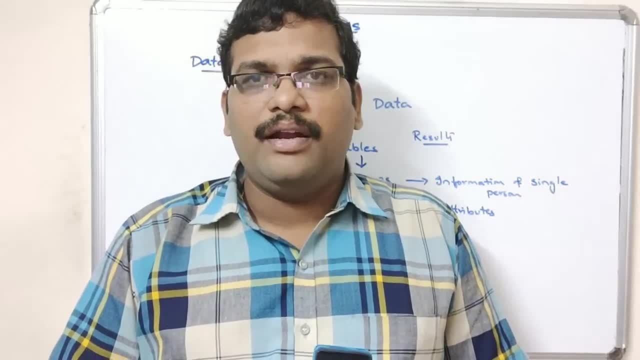 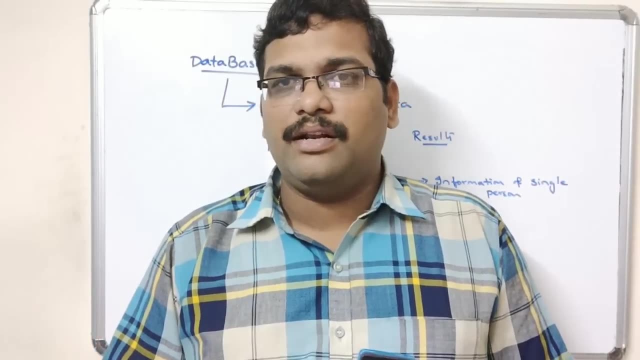 So definitely, I will try to clarify all your doubts And if you really understood my sessions like my session, share my sessions with your friends and don't forget to subscribe to our channel. Thanks for watching. Thank you very much.